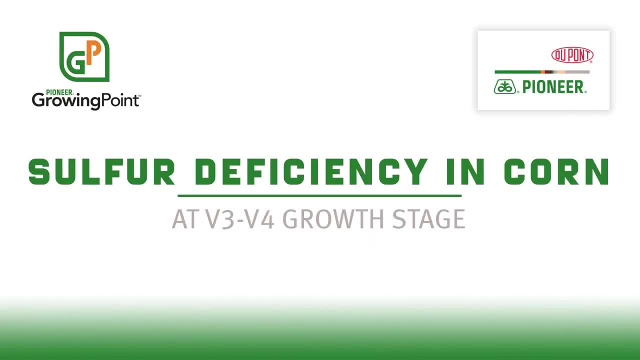 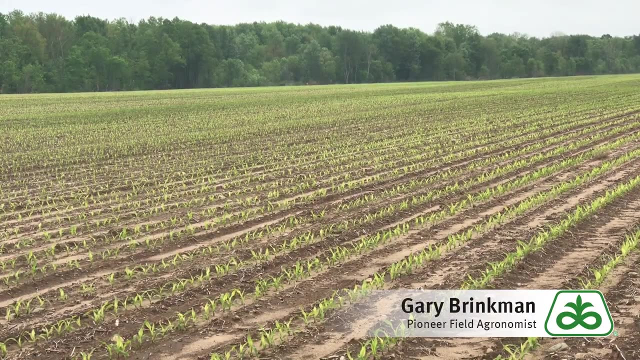 It's that time of year when we start to get the phone calls and growers are asking what is going on. in my field This is a great example. This field is right at that transition into V3 to V4. We're moving from the seminal radical roots into the nodal roots And that is the time that we often see transition colors. 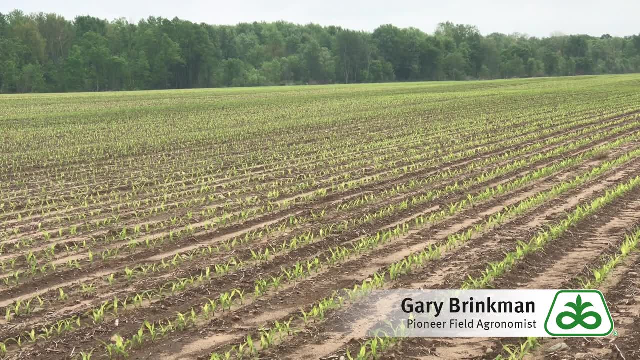 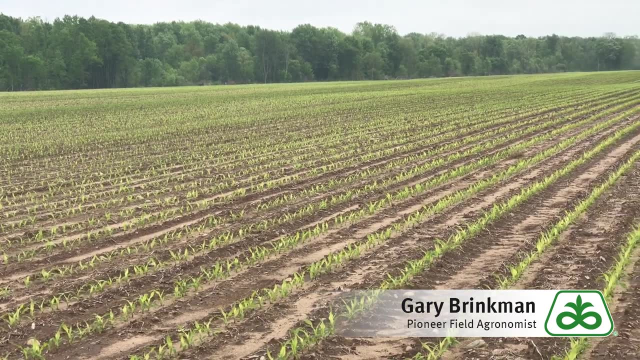 Slight differences in fertility soil types create some of those issues. This is a great example. As we look across this field here we start to see a dark green. We see a lot of very, very pale colored corn. So what's going on? 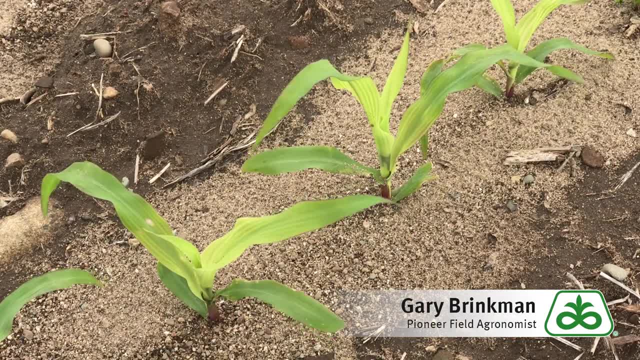 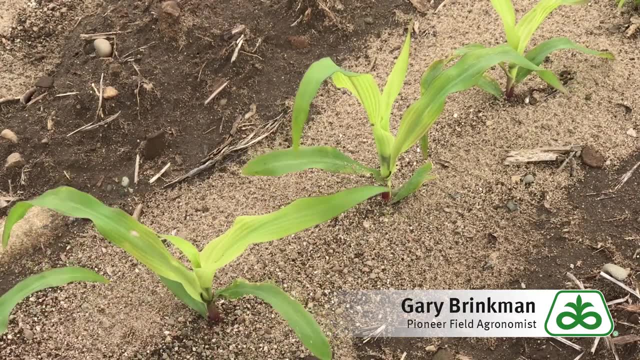 As we take a closer look at this corn. as I say, we're in the V3. We have one, two, three full colors that are starting to show almost V3. And this is a time when we start to see transition colors. 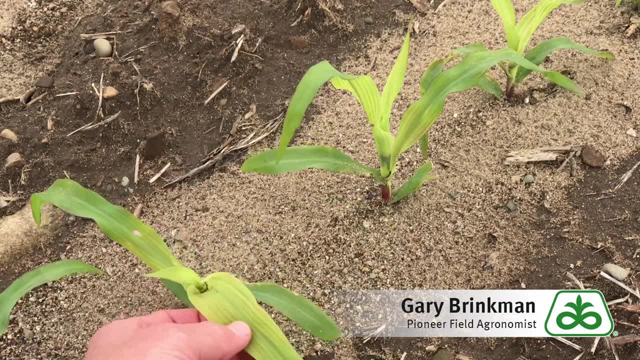 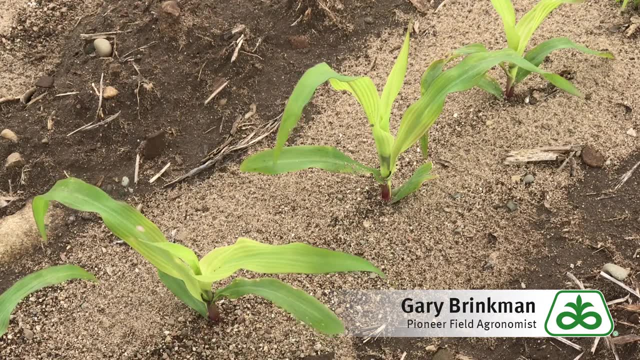 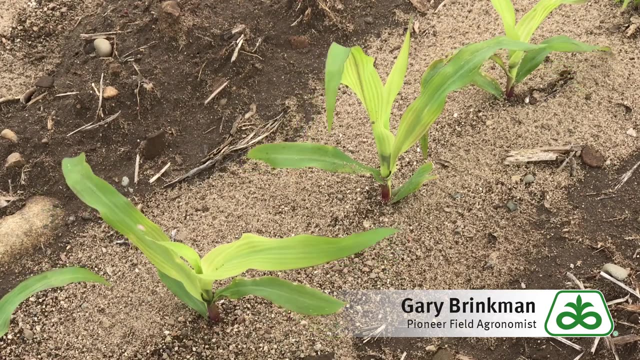 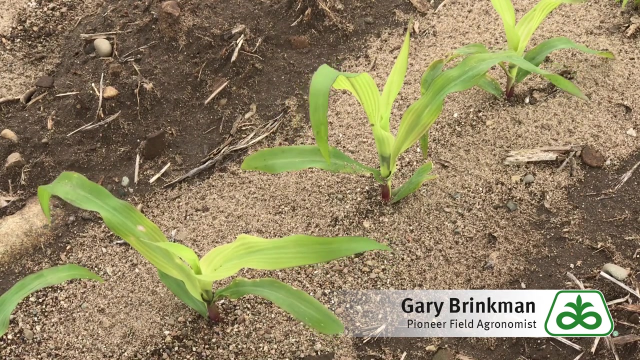 The plants that we see here. we see a lot of interveinal chlorosis, especially in the upper portion of the plant, the growing point Most likely with this sandy soil, we're looking at some sulfur deficiency. This could be a result. we've had some heavy rain through this part of the state. This could be a result of that heavy rain pushing the sulfate ion out of the root zone and temporarily causing some sulfur deficiencies. 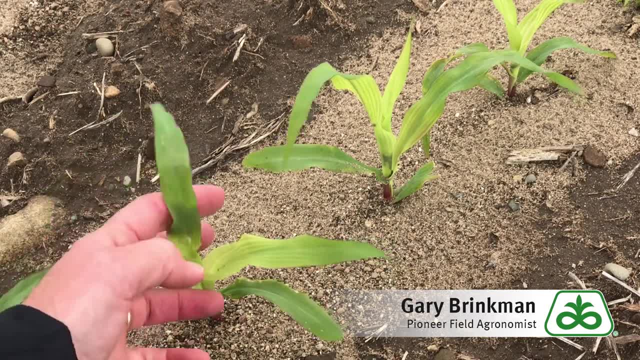 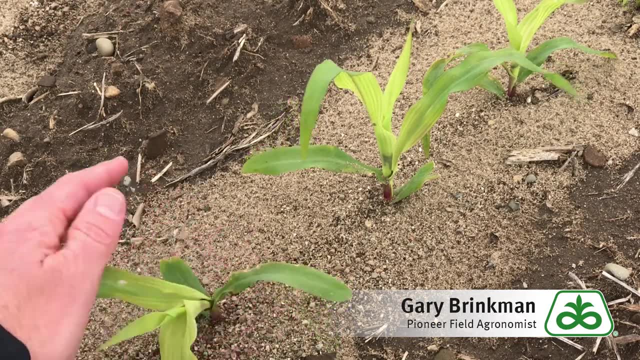 How do I know this is sulfur? Well, typically, if we look at a plant, the lower leaves will tell us whether it's nitrogen. Nitrogen deficiencies will show up in these lower leaves first, whereas sulfur deficiencies start to show up in the growing point and in the midsection of the plant. 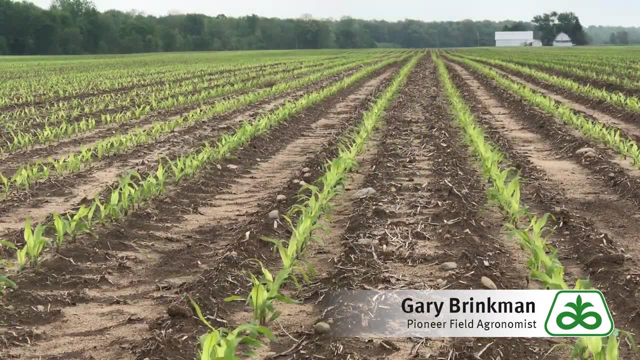 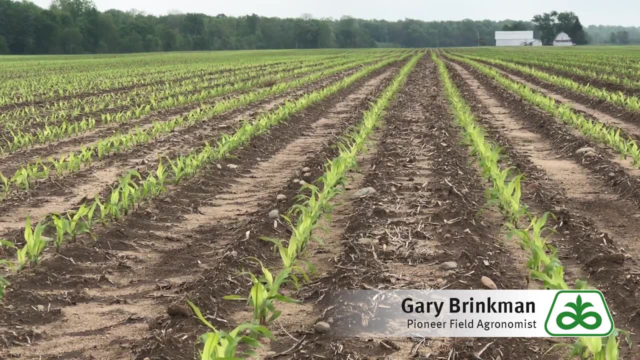 As we look down the row we can see that it's pretty consistent across the whole field. There are some areas where probably a little bit higher organic matter We're not seeing quite the distribution. We're seeing some discoloration, the chlorotic plant color, and there's probably some residual sulfur there. 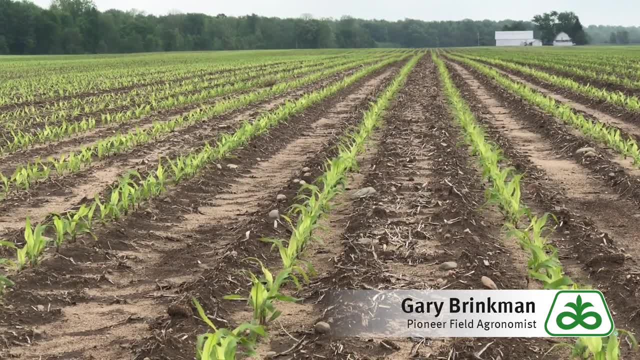 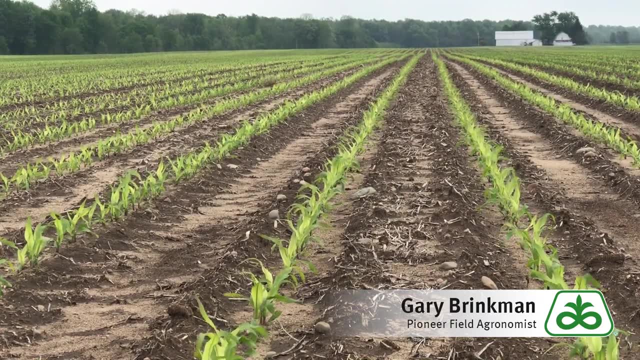 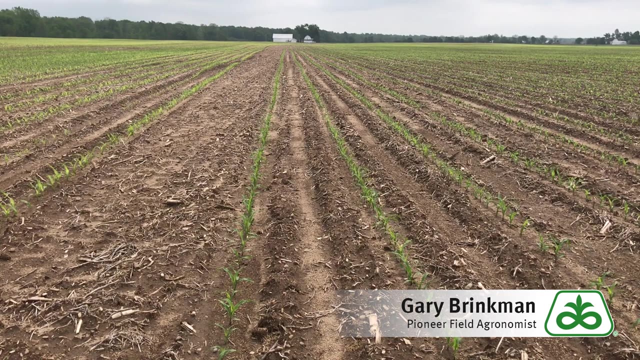 Now, the grower may or may not have used some sulfur in his starter, and certainly that would be one way that we can help alleviate some of these early symptoms of temporary sulfur deficiency. It just so happened that we have a part of the field where two different plantings took place.